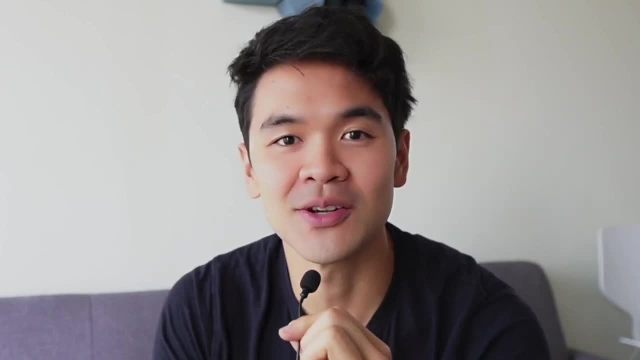 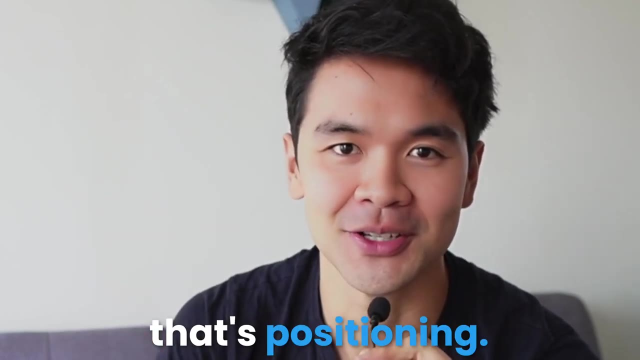 into is dirty. you just got to jump at that point. People will be in so much pain that they will buy in the first solution that comes to mind being that first solution that comes to mind. that's positioning, And that's what we're going to cover today. 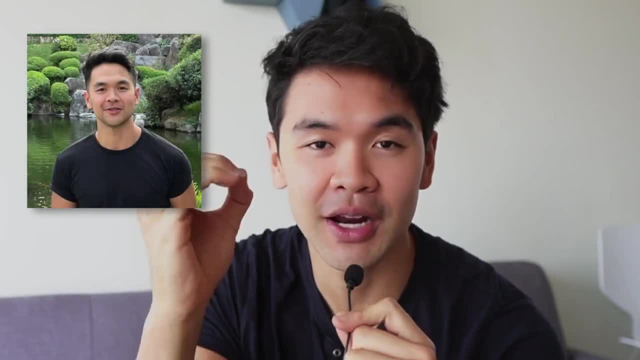 So that when people have that pain, the first person they think about is you and they'll show up to your door with their credit card and they'll just give you money And once you understand this, you're going to make a lot of money. 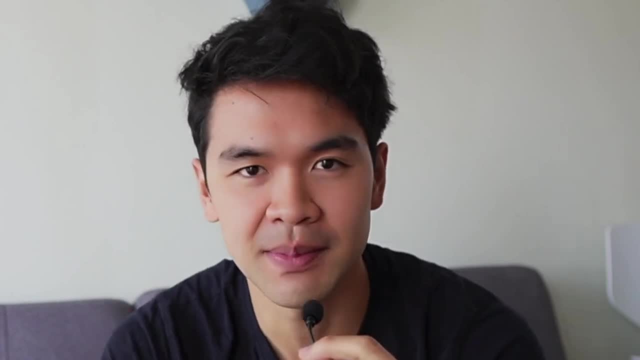 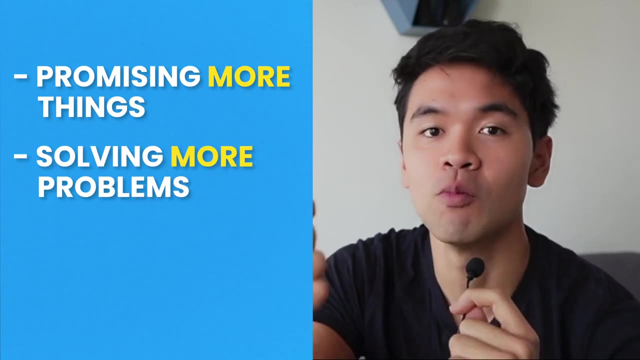 So let's get to it. There are two Paths you can take to be the best. The first one is to become the best by addition. You become the best by addition, by promising more things, by solving more problems, by solving bigger problems. 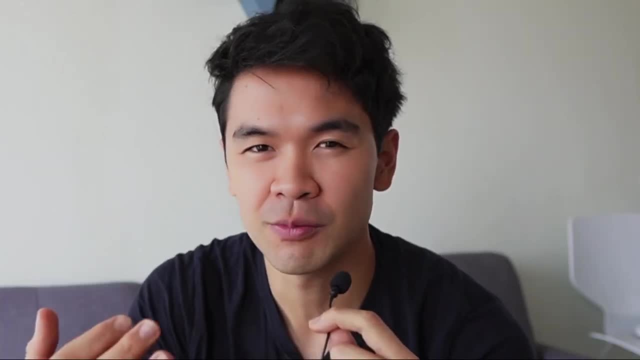 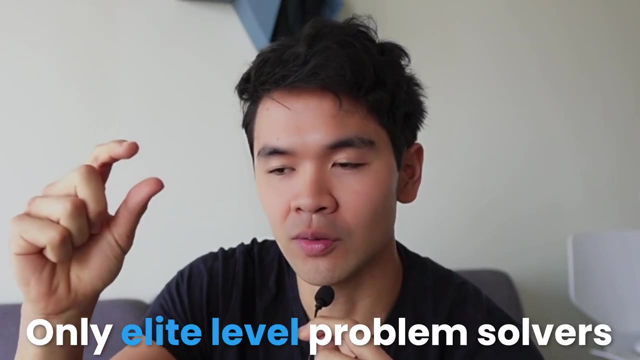 I don't recommend this. At some point, you end up in a position in which you solve many problems at a good enough level, but not one, and at a lid level and only a lead level. problem solvers take space in people's minds. Instead, I recommend becoming the best by subtraction. 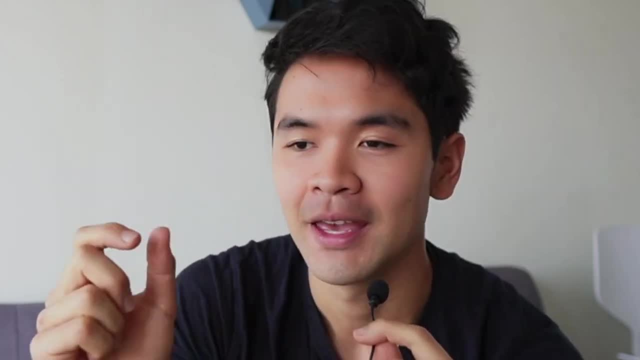 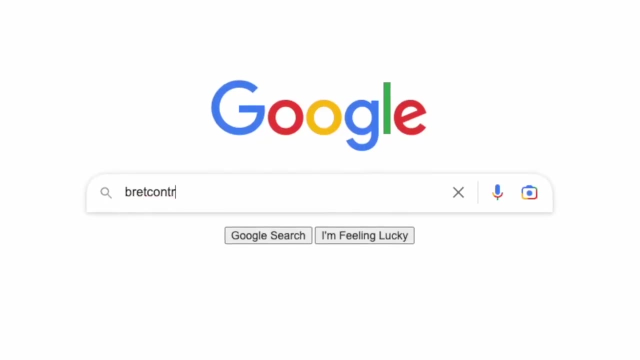 Subtraction is solving the last problems, but solving them better, And the best example I can think about of this is fitness coach Brett Contreras. So Brett Contreras is known as the glue guy, But if you go to his website, you'll find an astounding number of ass. 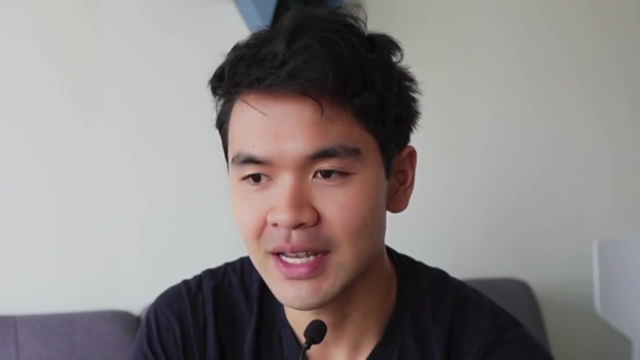 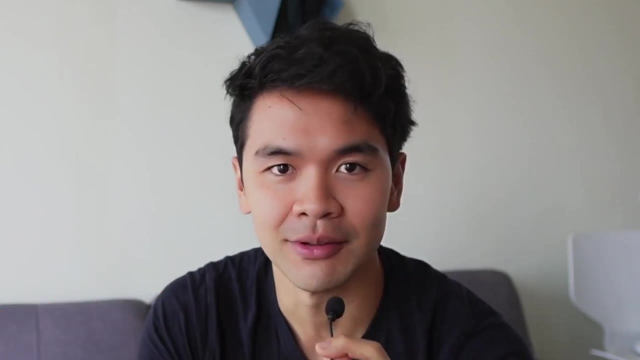 Like you'll just find a lot of glutes, because he is the glue guy. He understands that there is more money in solving a smaller problem at an elite level than solving many problems at an okay level, And he's worth $50 million. 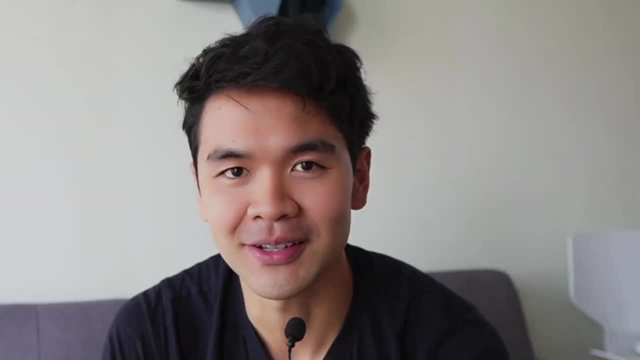 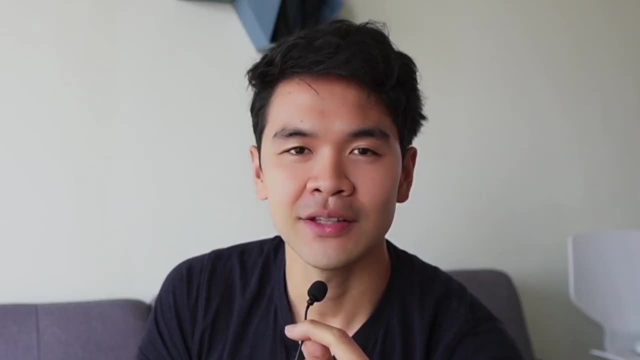 So something's clearly working. Then you encounter kind of a paradox: How do you find a problem that's small enough so you can be the best At solving it, But that's also big enough so that it's profitable And to solve that? let's say you're a tour guide. 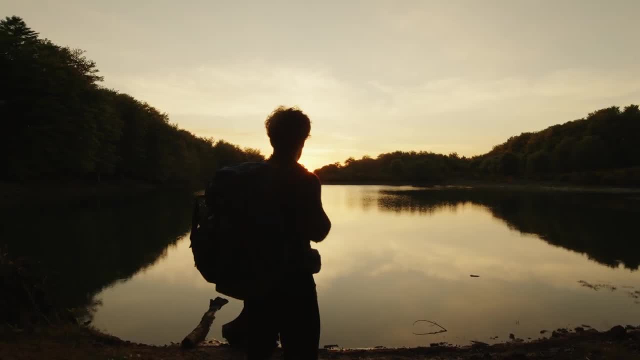 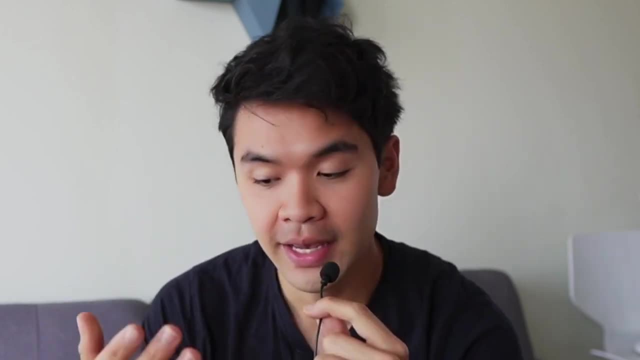 You take people through tours in the forest and you belong to a tour company. People come to the tour company and they say, hey, we'd like to tour for the forest, And the lady at the front desk says no problem, Hands in my brochure and the brochure. 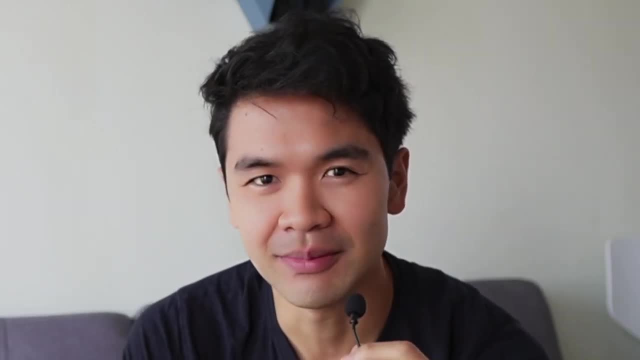 It's you and all the other tour guides, But they all kind of look the same. They promise almost the same thing. It's the same path, some perks here and there. So what they do is they don't really want to think about it. 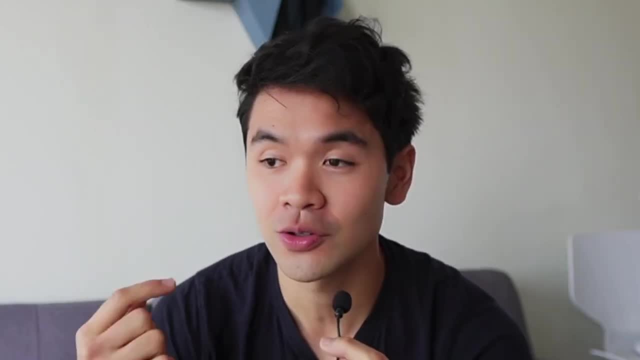 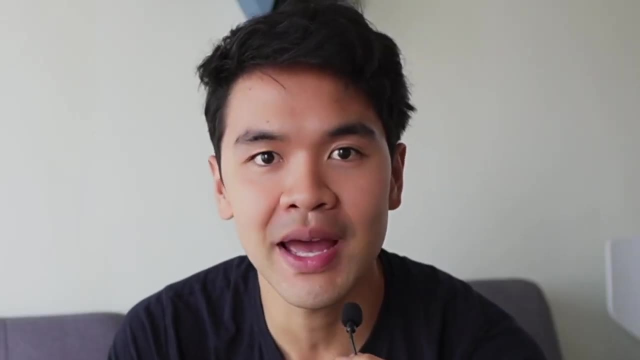 So they just choose the one with the best track record, And that's not you. So you realize that. but you're smart about it. You go to the forest the next day and you trailblaze and you find where can you get new paths. 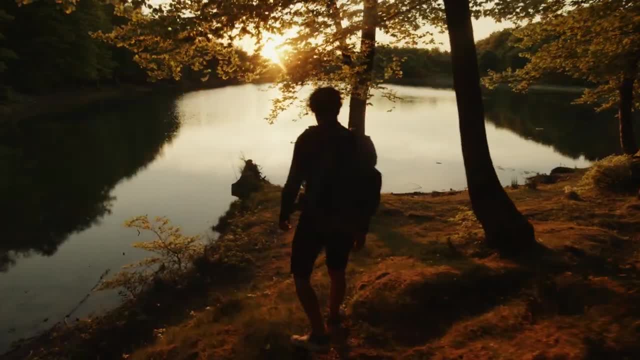 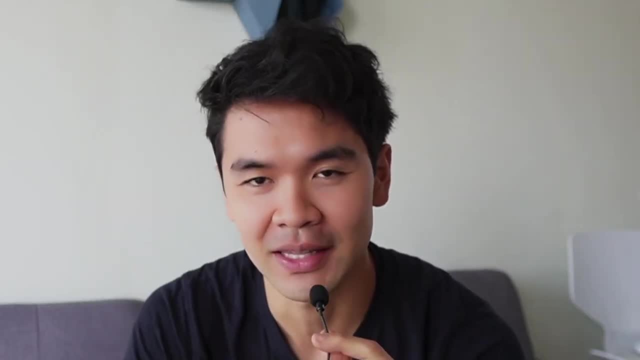 You find one that has its pros and cons. It's not the best thing in the world, but you found one and nobody knows it exists, Just you, which means you are the best at finding that path. The important thing to note here is that everybody promises the same thing. 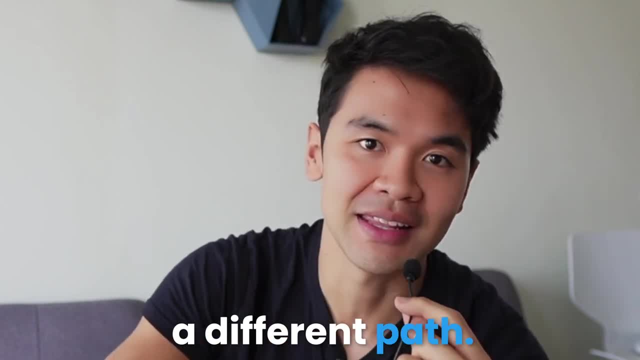 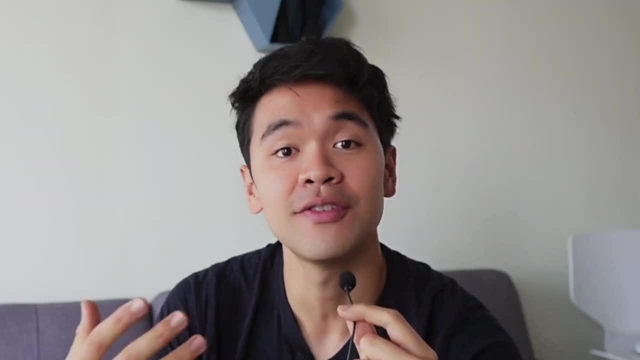 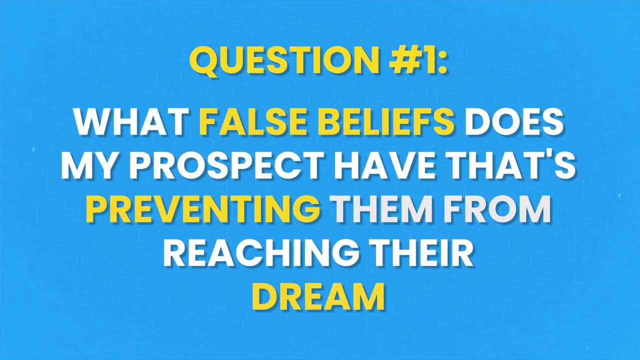 You don't promise anything different, but you promise a different path, And off that path you're the best one because you're the only one that knows it. My favorite two questions to ask myself to find different paths are as follows: What false beliefs does my prospect have that's preventing them from reaching their dream outcome? 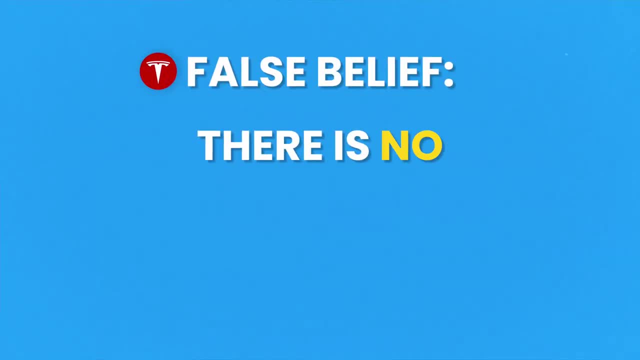 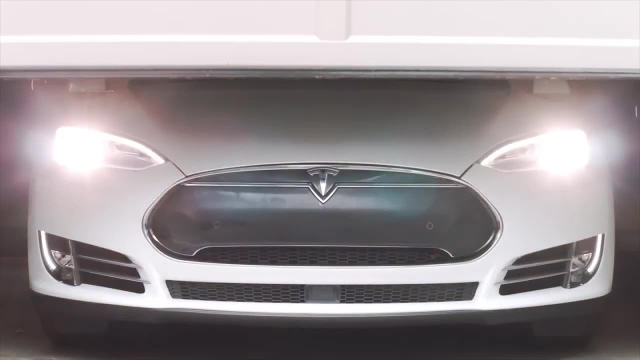 Tesla right. The false belief they're tackling is there is no way to have clean energy that's not extremely expensive. So Tesla comes in. they come up with an electric car that doesn't pollute the planet but also doesn't break the bank. 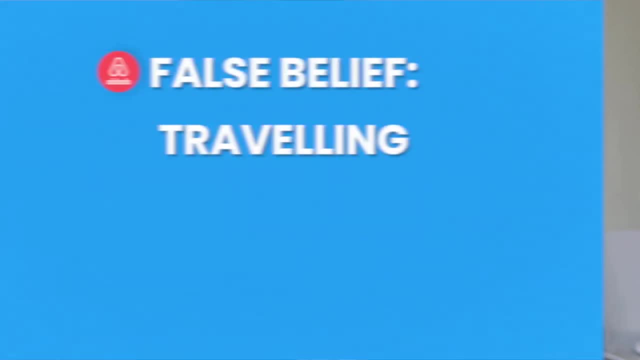 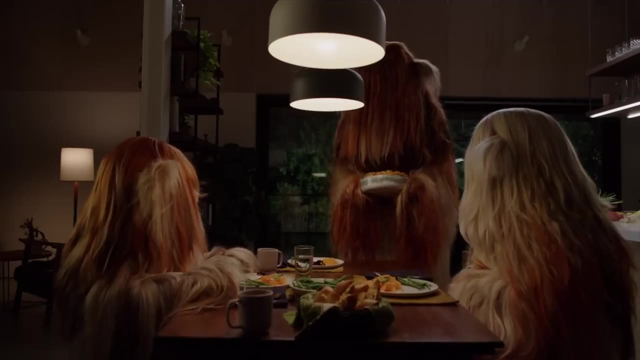 Two is Airbnb. The false belief they're tackling is traveling is a lot of money because I have to spend it in hotels. So they come in And they say actually you don't, You can just stay with local and save money that way. 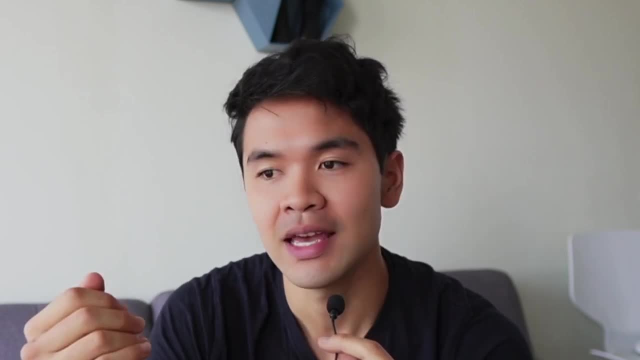 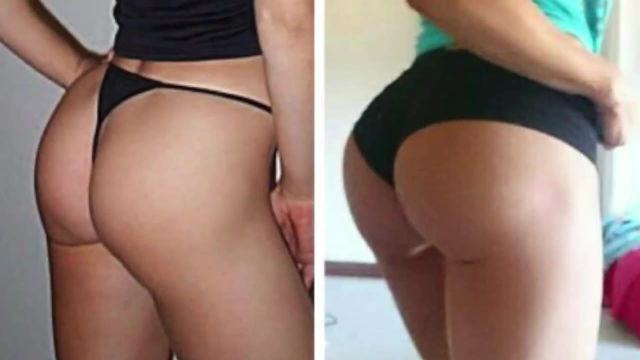 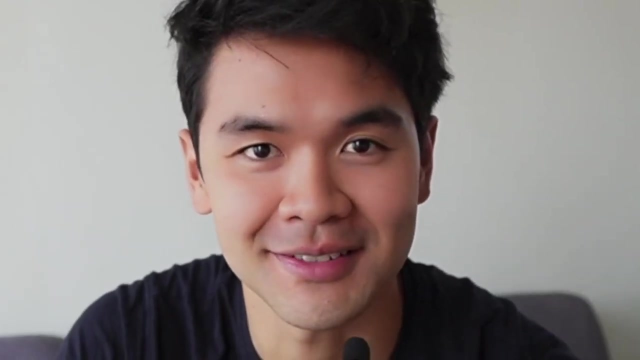 And the second way I like to think about how to find a different path is missing pieces. What missing pieces can I fill in so that they can get to their dream outcome? So bread promises you you'll get the body you want, But the missing piece you have is, if the body part you care more about is your ass, will just, you know, train your ass? 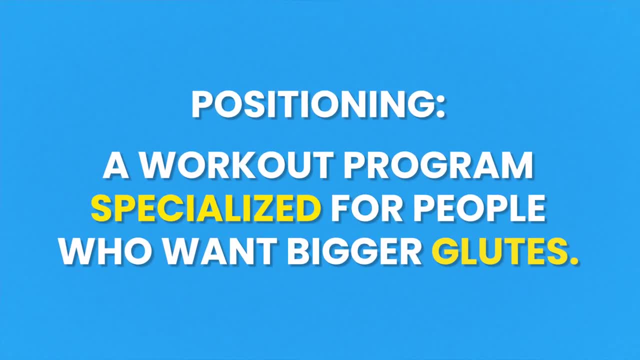 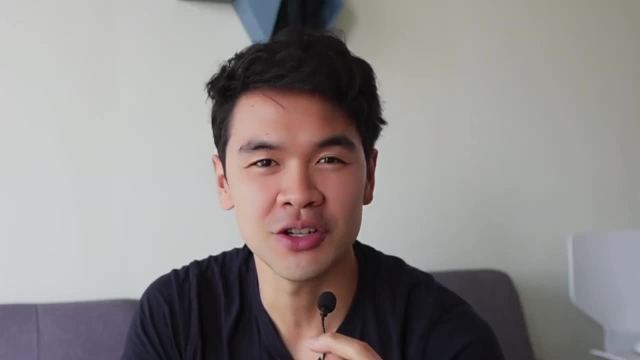 So his positioning is a workout program specialized for people who want bigger glutes. It's so funny, but it's so effective, God. second one is Grammarly. Maybe you write a lot, but your English isn't the best. English is your second language. 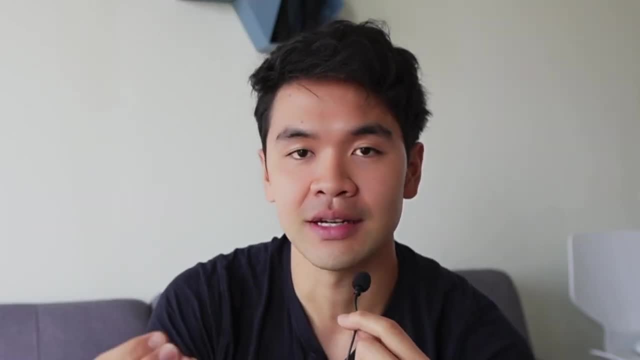 You know, like me, I use Grammarly a lot, So Grammarly fills in as the missing piece and tells you: you do your thing. You just write will correct you along the way. Airbnb doesn't give you the best staying experience. 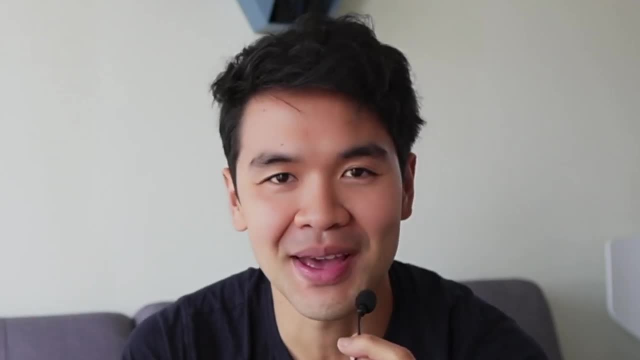 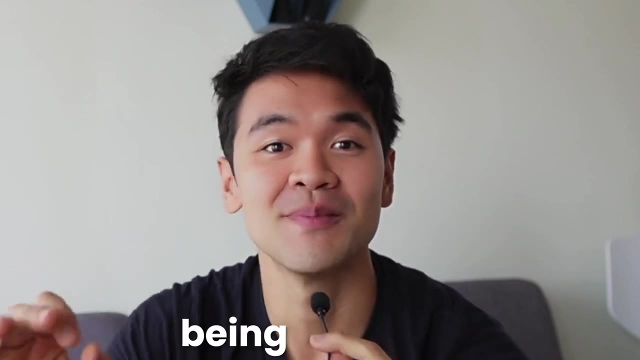 Tesla doesn't give you the best driving experience, But that doesn't matter, because they understand one very simple truth that I'd like you to understand as well, which is: you're not in the business of being the best, You're in the business of being the only. 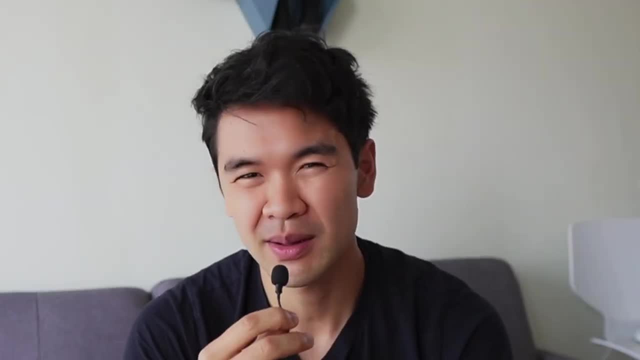 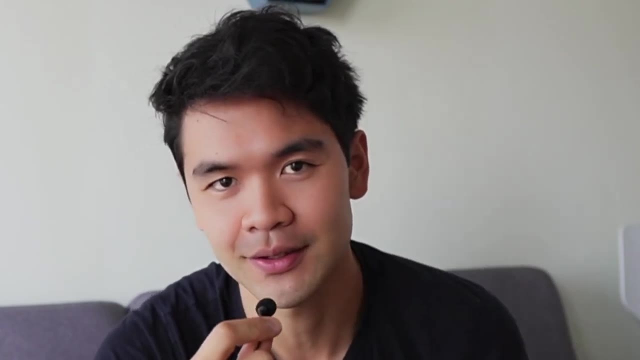 So let's take it back to marketing. Marcos is a ghostwriter, And if you know anything about Ghostwriting on Twitter is that there's thousands of people that promise ghostwriting and they all kind of promise the same thing And at some point it gets ridiculous. 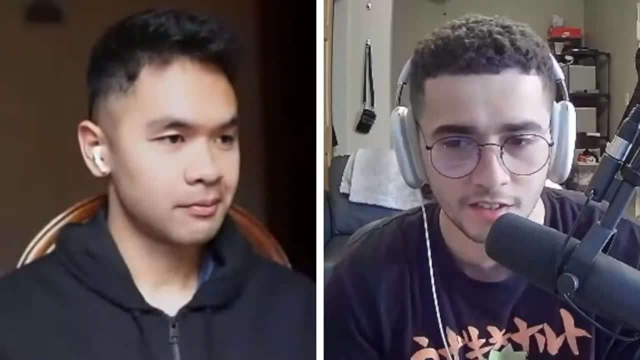 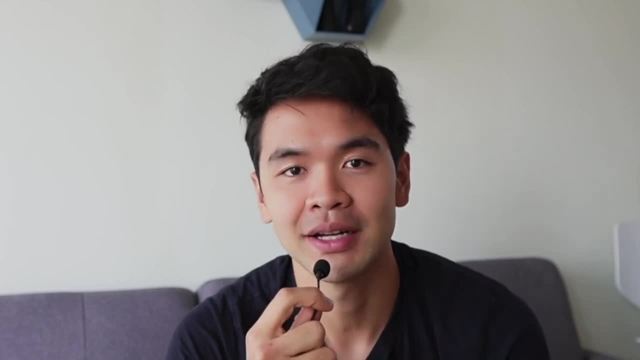 Marcus saw this and he said: there's no way I can compete with people that have 100,000 followers and promise ghostwriting, Like they just have so much more credibility than me. So what he did is screw growth. I'm the monetization ghostwriter- the ghostwriter for people who are more interested in building a business than building an audience. 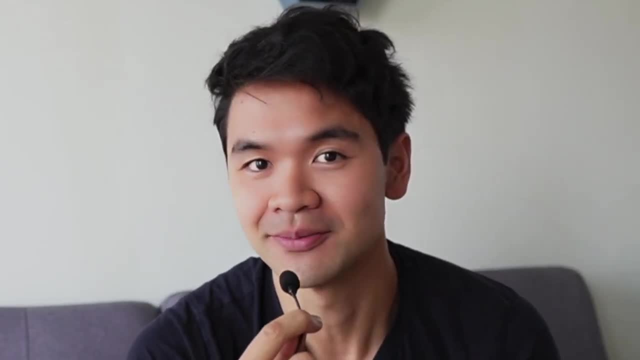 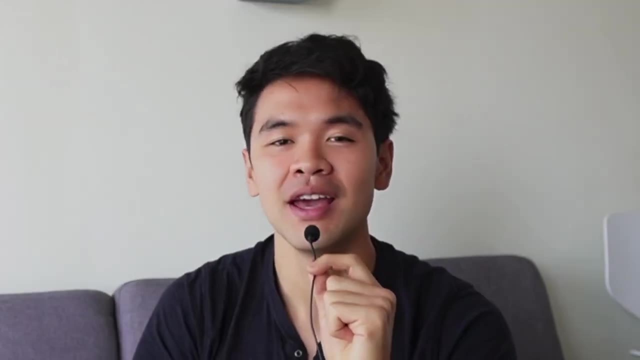 And he's making $30,000 with 11,000 followers. So something's working. So how do you find your unique positioning? now It's your turn. So first thing is, you got to find your dream outcome and don't get too caught up here. 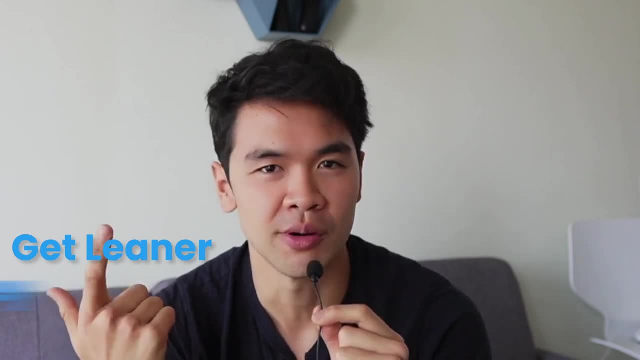 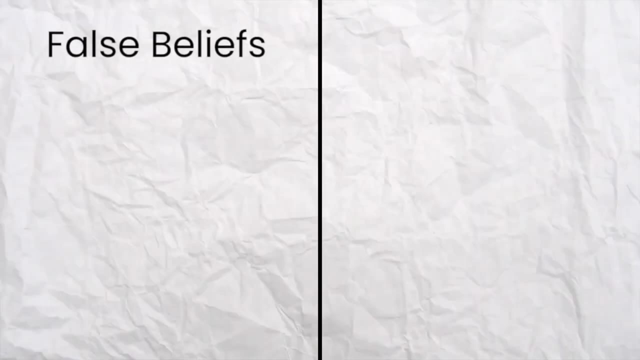 People kind of want the same things. They just want to get leaner, They just want more money and they just want better relationships. Like, don't get too deep into this. Take a piece of paper and split it in half. In one side you're going to write false beliefs, and then the other side you're going to write missing pieces and then write as many as you can. 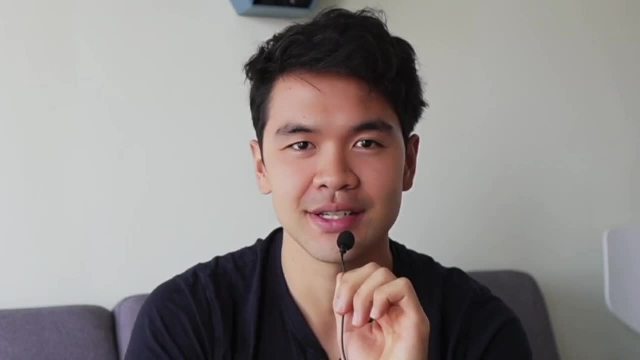 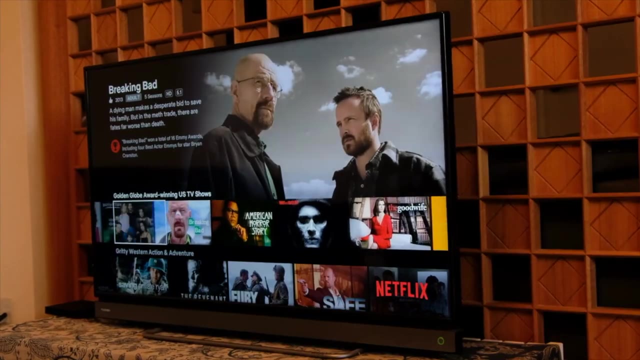 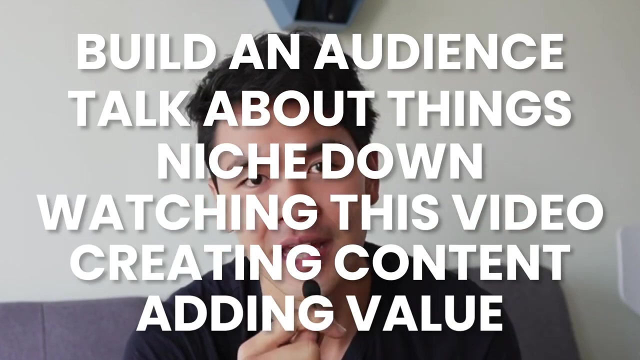 Just go ham Like you should have 10,, 15,, 20 on each side. So all these false beliefs and missing pieces occur to you for a reason. There's a reason besides the money That you don't sit and watch Netflix all day, that you actually build an audience and talk about things and niche down and you're watching this video and create content and add value. 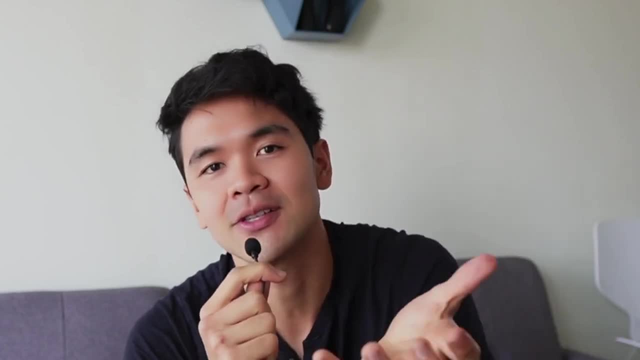 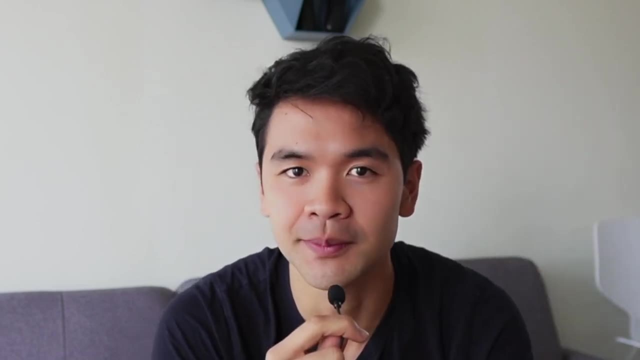 Because at some point in that amalgamation of stuff, you found something that really helped you, And this is why you wrote the false beliefs and the missing pieces that you wrote, because it really helped you. And what you got to do is you got to read through those and think which one of these has helped me the most. 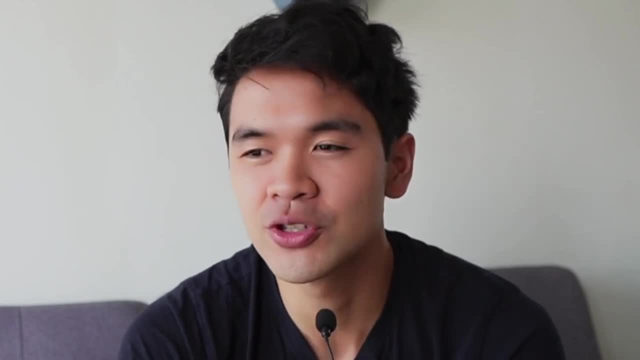 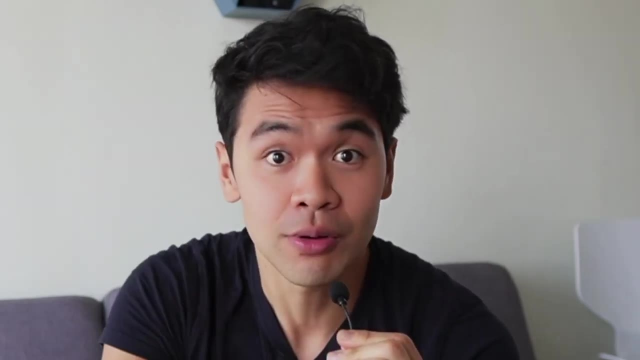 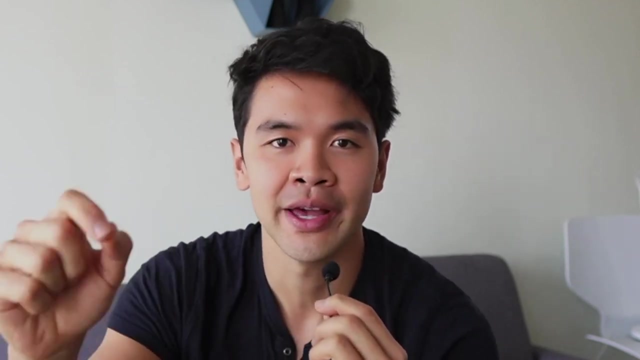 And eventually, when you find one, it'll feel different. It will just feel like this is right And this is what you want people to feel, because then you'll have evidence that it works. You are the evidence that it worked And you also have the belief and the conviction that, if it helped you, you can use that gift to also help others. 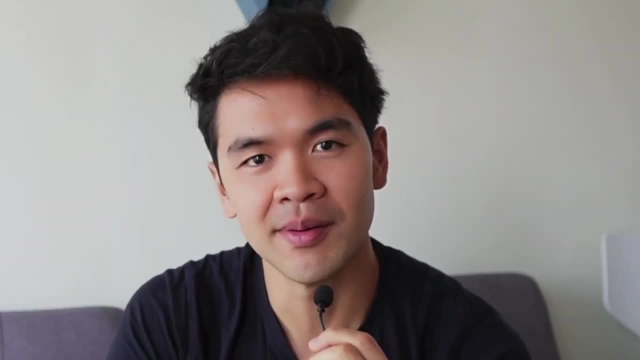 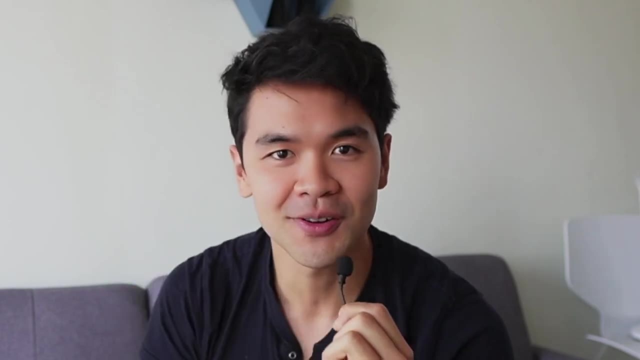 And that's how you position yourself. You find a false belief or a missing piece that really helped you, And when you find one, you just say that 1000 times until people start believing it, which is also known as my Twitter strategy. 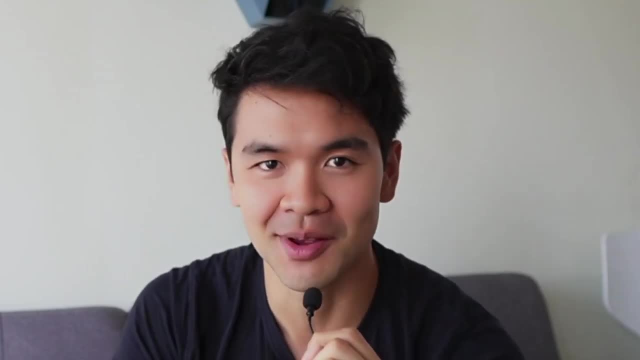 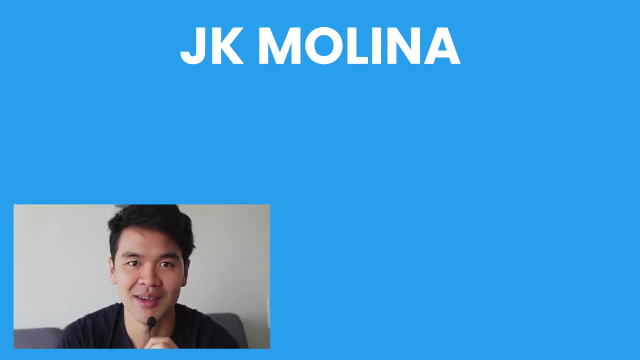 I'll just say likes in cash, 10,000 times every month and somehow it's working, So hopefully It also works for you. Hope this video worked for you. If you want to grow your audience, I'm not your guy, But if you want to monetize your audience, you can subscribe to the channel and watch the other videos. And remember likes in cash.